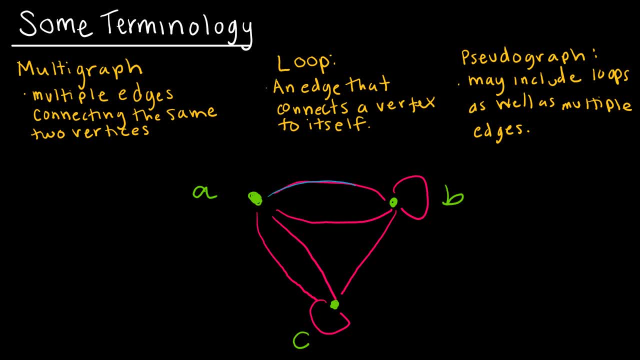 or connecting the same two vertices. So here I've got an edge connecting A B and here I have another edge connecting A B, and that's what makes this a multigraph. A loop is a loop that connects two vertices. So if I had an edge connecting A B and here I have, 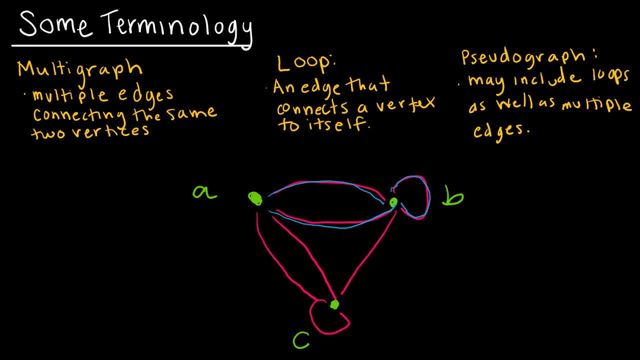 a loop. however- again, we talked about that a little bit- A loop connects a vertex to itself. A multigraph actually would not contain any of those loops, but a pseudograph is what I have pictured here, which contains both multiple edges and loops, So it could include one or both. 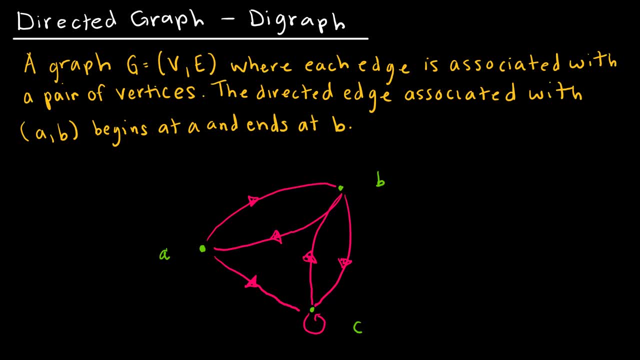 We've already spoken a little bit about digraphs, but I'm going to talk a little bit more about the directed graphs. And this is just a graph where each edge is associated with a pair of vertices. So the directed edge associated with A, B begins at A and ends in B, etc. So if we were to list, 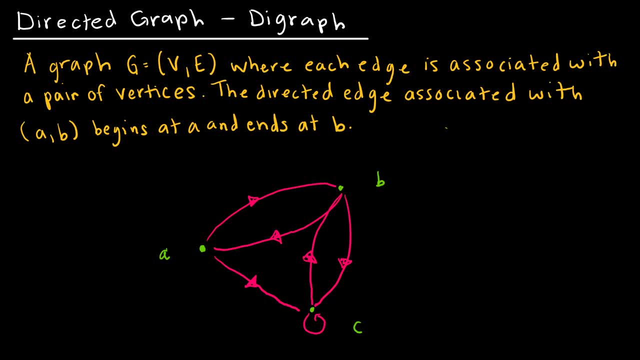 the vertices included in this directed graph, we would have A- B because A goes to B. So I've used this one And I would also have A C because A goes to C. And then, looking at the directed graph, we would have A- B because A goes to B. And then, looking at the directed graph, we would have A- B because A goes to B. 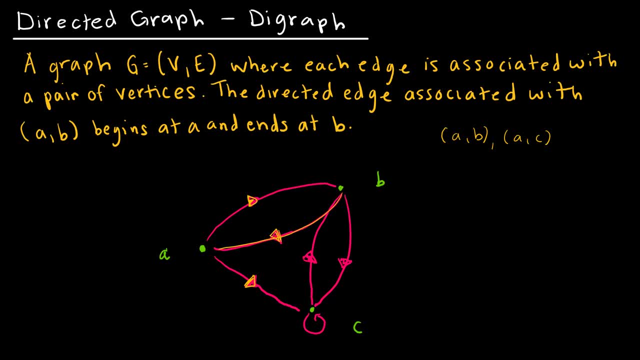 And then, looking at the directed graph, we would have A- B, because A goes to B. I've got one from B to A, So B- A would be two points here: B to C And then from C. I have C to B And I also have C unto itself. 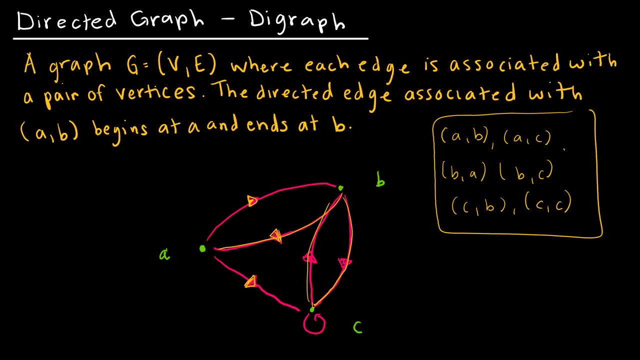 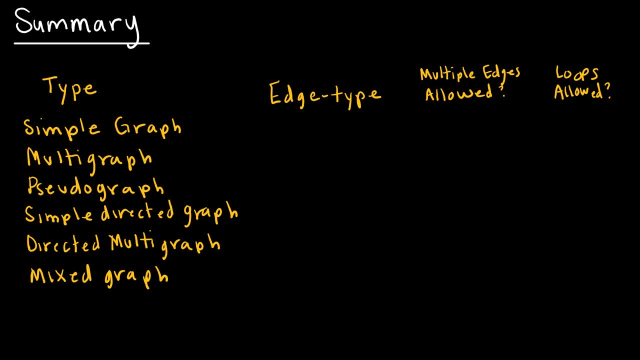 So these would be the ordered pairs that would be associated with this particular directed graph. So just a quick summary: we have simple graphs, multigraphs, pseudographs, a simple directed graph, which we didn't speak about in specifics, a directed multigraph and a mixed graph. So let's talk about what. 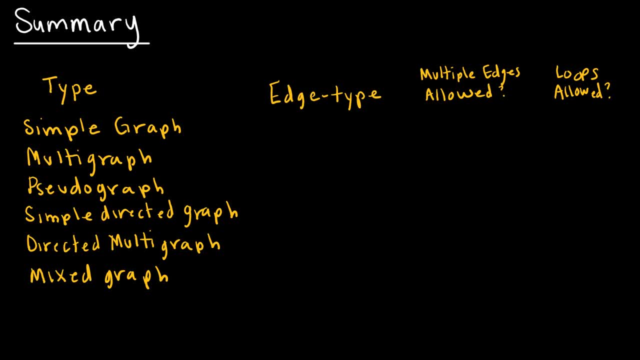 all of those things are. We know a simple graph has edges that are not directed, And does that allow for multiple edges? No, because it's simple. Can you have a loop in a simple graph? No, you can't again because it is simple. But if we're looking at a multigraph, 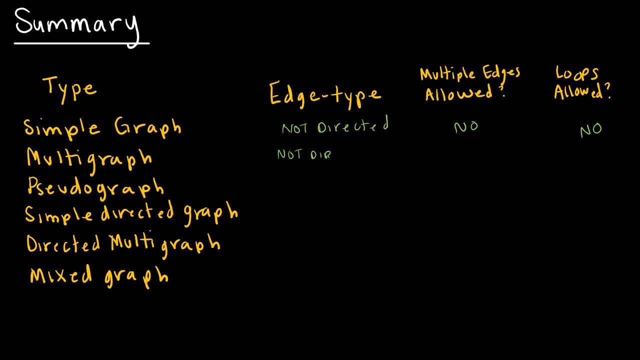 a multigraph still has not directed, so it's non-directional. I can have multiple edges, but I still cannot have loops. So if I want this to be a yes in a non-directed graph, then it's got to be a pseudograph I can have. multiple edges, but I still cannot have loops. So if I want this to be a yes in a non-directed graph, then it's got to be a pseudograph. I can have multiple edges, but I still cannot have loops. So I can have multiple edges, but I still cannot have loops. So if I want this to be a yes in a 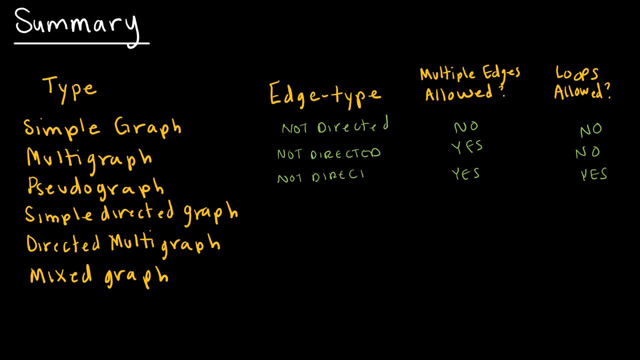 non-directed graph, then it's got to be a pseudograph. Again, this is not directed. So now let's talk about directed graphs. So we just sort of threw it out there, but I didn't talk about any specifics in the directed graph. So there is such a thing as a 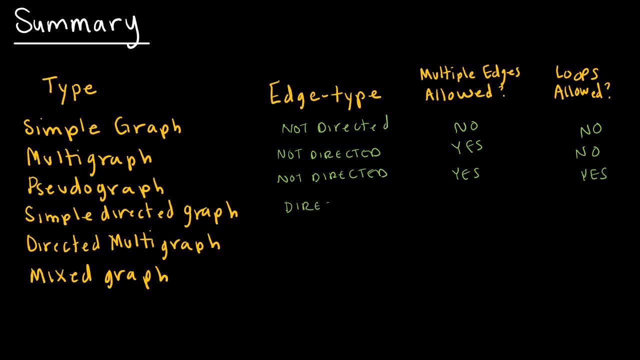 simple directed graph which of course would be directed here for the edge type, But because it is simple, again, we would not have multiple edges or loops allowed. If I look at a directed multigraph, a directed multigraph again does have directed edges. 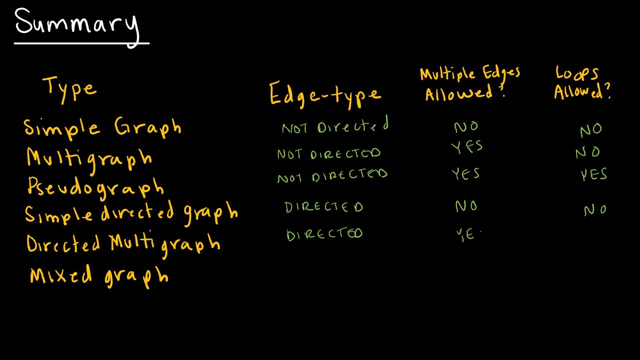 And because it's a multigraph- yes, we can have multiple edges. And because it is directed- yes, we can also have loops on a directed multigraph. And a mixed graph essentially gives us the opportunity to have some edges that are directed and some edges that are not directed. 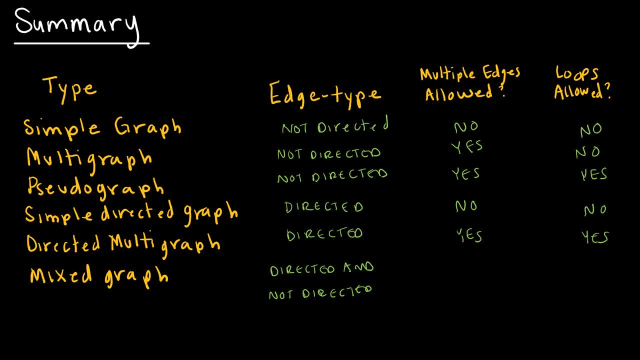 So we can use either, or because it is a mixed graph. We're essentially saying: you know, go to town, you do you? Multiple edges allowed- yes, Yes, they are. Loops allowed- yes, they are. So that's sort of a quick summary of the types of graphs that we've been introduced to. 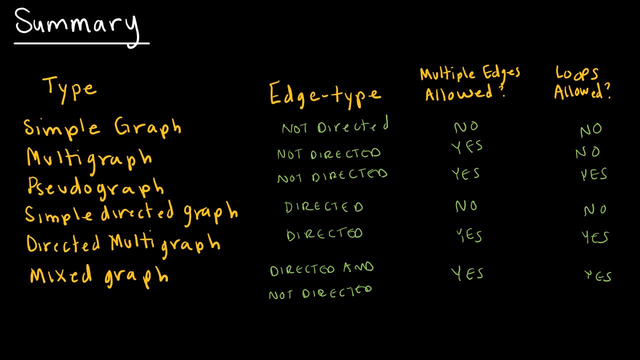 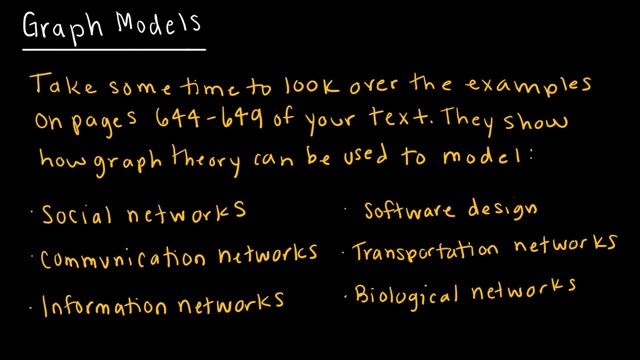 We're going to spend quite a bit more time on graphs in our next lesson, So this was just a brief introduction. I did not go through all of the graph models, So your textbook does a great job of talking about some of the different ways that we can use graph theory in social networks, communication networks.